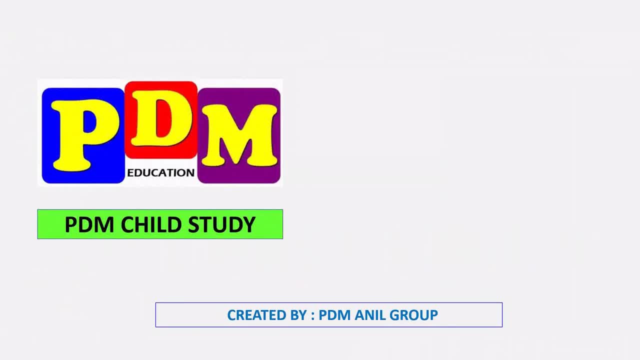 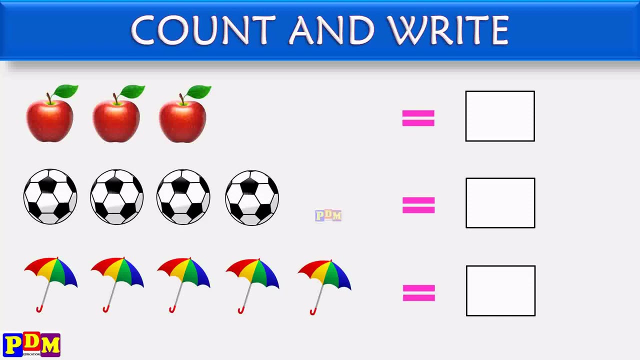 PDM Child Study. Subscribe our channel for more educational videos. Count and write: 1 2, 3 Is equal to 3. 1, 2, 3. 4 Is equal to 4. 1, 2, 3, 4, 5. 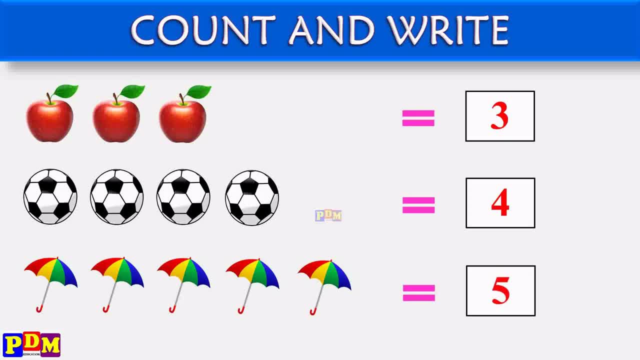 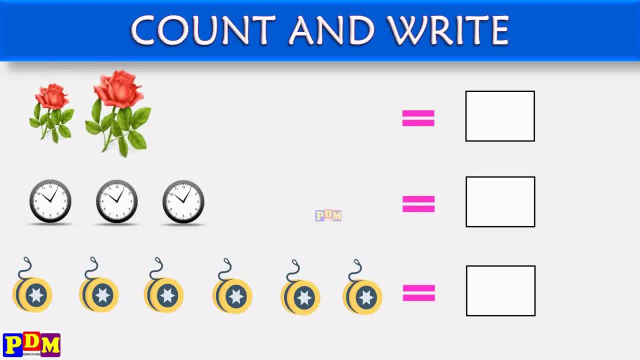 Is equal to 5. 1. 2 Is equal to 2. 1, 2, 3, 4, 5, 4, 5, 6, 7, 8, 8, 9, 10, 11, 12, 13, 14, 14, 14. 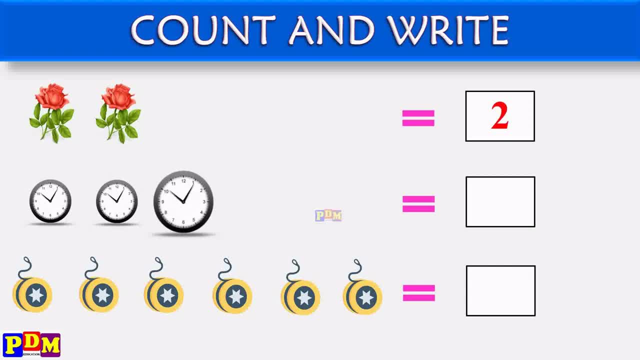 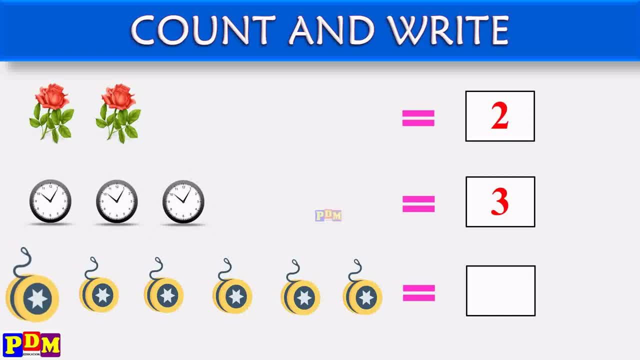 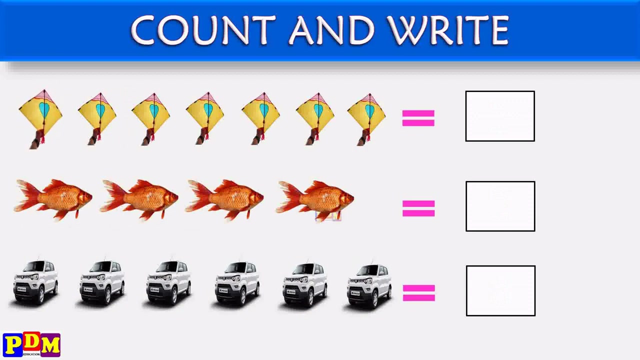 47, 47, 49, 51, 51, 52, 52, 53, 52, 53, 54, 55, 56, 67, 67, 68, 68, 69, 69, 70, 71, 72, 72, 73, 73, 74. 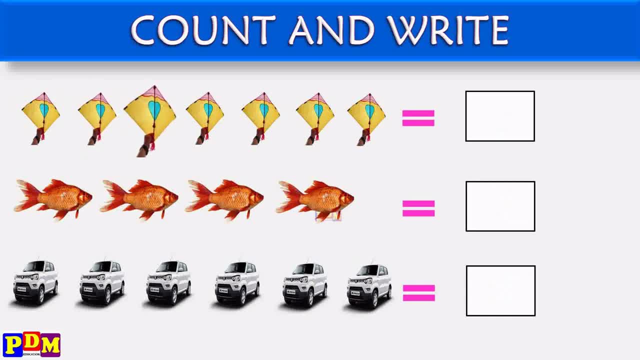 74, 75, 76, 76, 77, 78, 78, 79, 89, 90, 91, 92, 93, 92, 93, 93, 94, 94, 95, 96, 97, 96, 97, 97, 98 98. 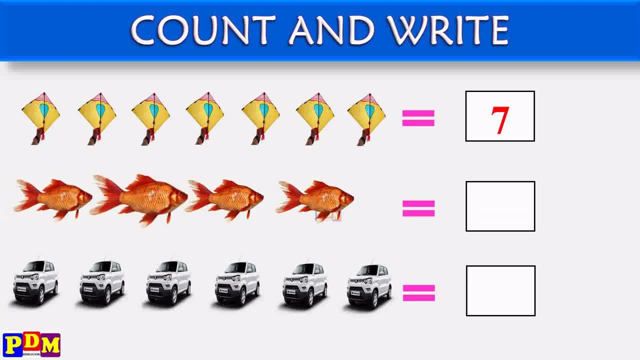 99, 100, 100, 12, 13, 14, 15, 16, 17, 18, 19, 20, 22, 23, 24, 25, 26, 27, 28, 28, 29, 30, 31, 32, 33, 32. 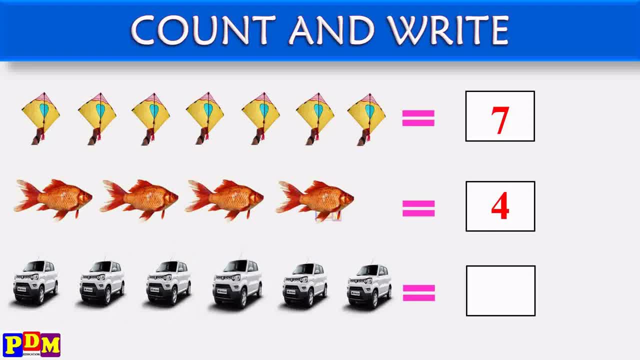 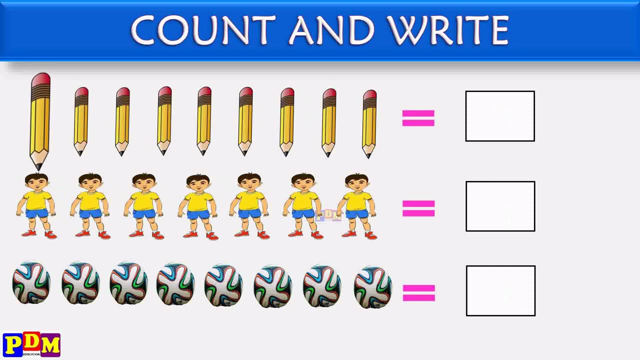 33, 34, 35, 36, 37, 38, 39, 40, 41, 42, 43, 44, 45, 46, 47, 48, 49, 49, 50, 51, 52, 53, 53, 54, 55, 56. 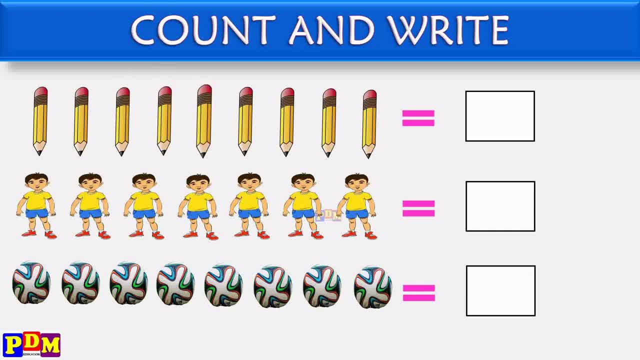 56, 57, 58, 59, 60, 61, 62, 63, 63, 64, 65, 67, 68, 69, 69, 70, 71, 72, 73, 74, 75, 76, 76, 77, 78, 79. 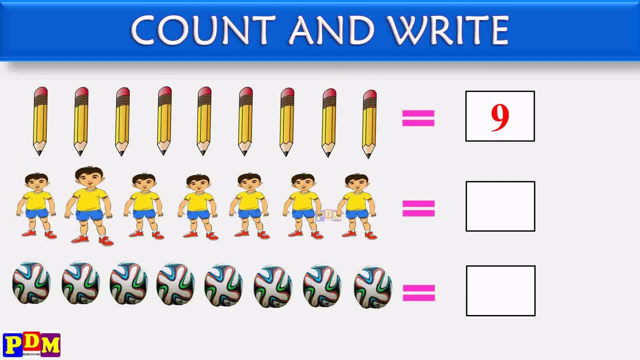 80, 81, 82, 83, 82, 83, 84, 85, 86, 87, 88, 89, 90, 91, 92, 93, 93, 94, 95, 96, 97, 97, 98, 99, 100, 100.